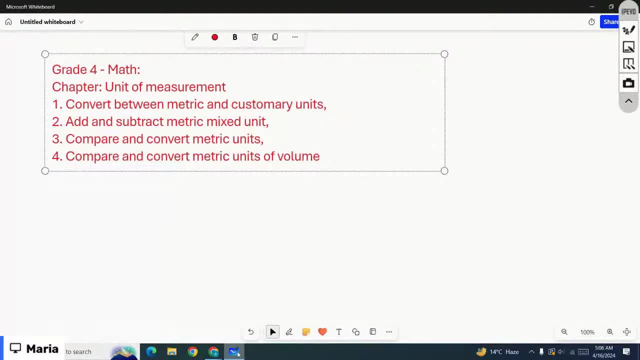 Hi everyone, hope you all are good. We are here for a grade 4 math. You can find all the lessons on ablestudentscom. You have to log in there using your email address and password as provided by the administrator. Then you have to select. 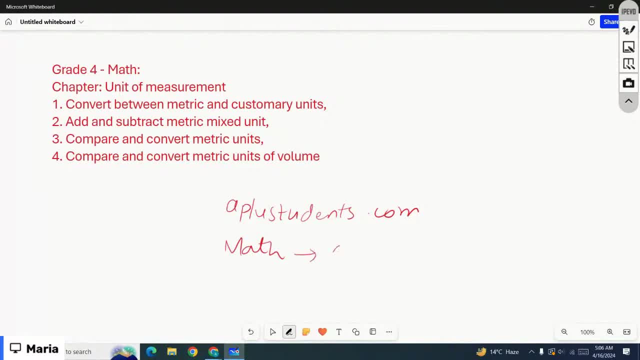 math from the subject tab, Scroll down to grade 4 and then click on view all lessons. There you can find a list of the chapters. We are going to start with the chapter unit of measurement, And the lessons we are going to cover today are: convert between metric. 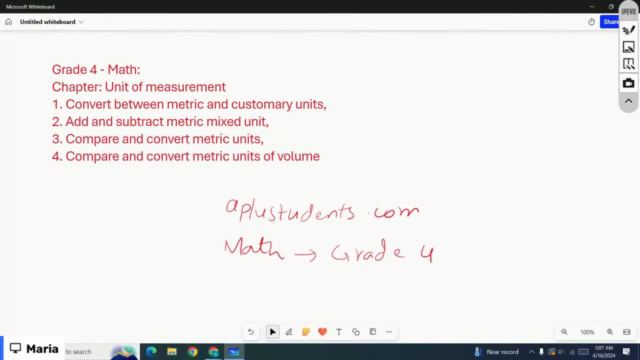 and customer units. add and subtract metric mixed unit, compare and convert metric units and compare and convert metric units of volume. So please make sure you have your notebook and pencil so that you can note down the important examples and definitions as well. So let's. 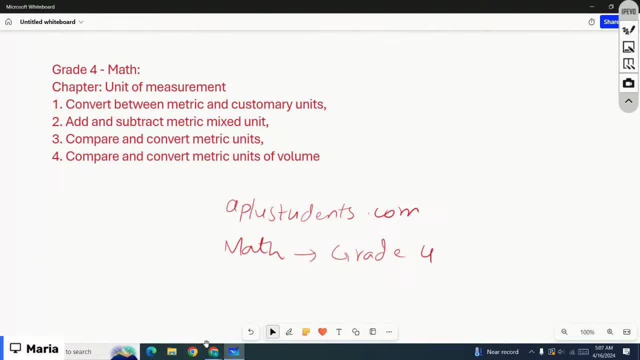 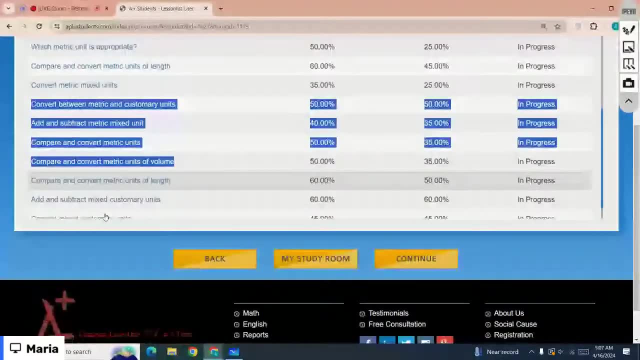 just start with the first lesson, that is, convert between metric and customer units. Here I am on grade 4 math. Let's just start with the first lesson, that is, convert between metric and mixed units. metric and customer units- Sorry, that was just a technical issue, that's. 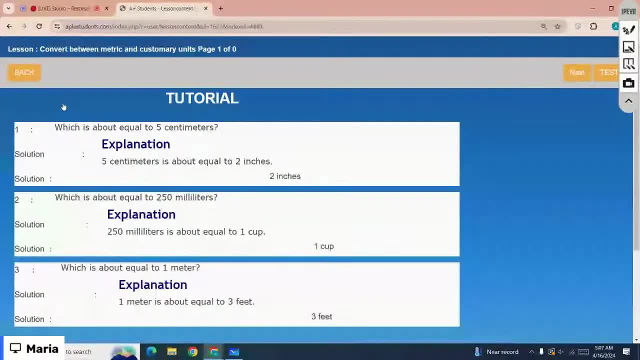 why the class is a bit late, right? So let's just start with the first example, that is, which is about equal to 5 centimeter. No, we were not done with the lesson. We have some lessons remaining from this chapter. Basically, I am already covered the I have already covered. 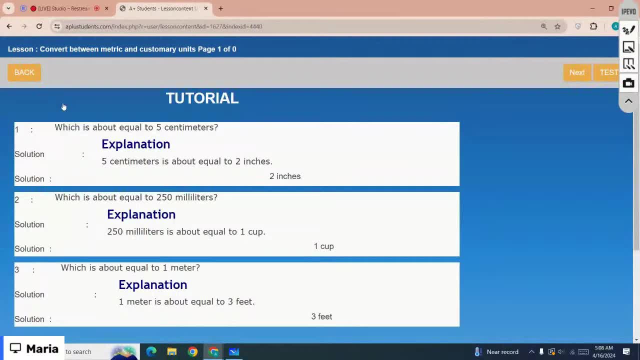 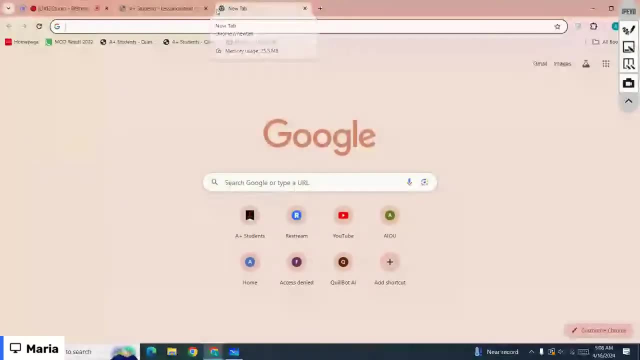 these lessons three, four times. that's why you did the lessons look the same. No, not the four time. how you did this four time, I am the one who is covering these lessons. let me show you. We are all going to see this little section. Oh, let me see some. 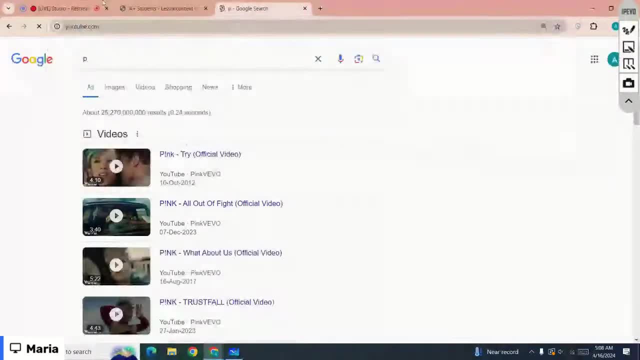 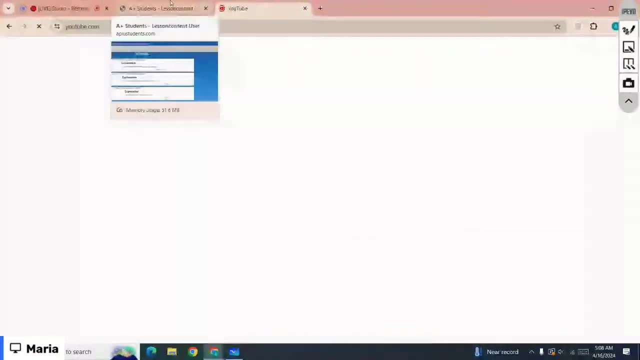 on math here. Actually, it's very difficult to come to station. hold on, let me just go to the channel. I will show you- I am the one who is covering the lessons daily- and how you. They are covered Here, at least they are today- How they are prepared. Okay, hold on. I remember last place you meet, some of view made a complaint that I am 아니. I'm notin temperament부. 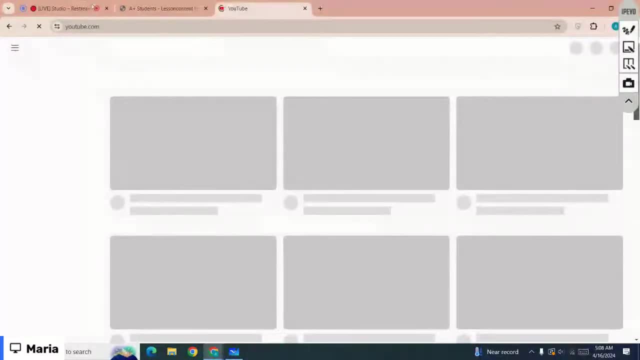 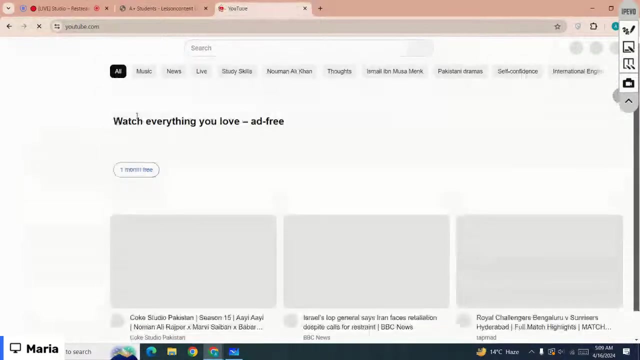 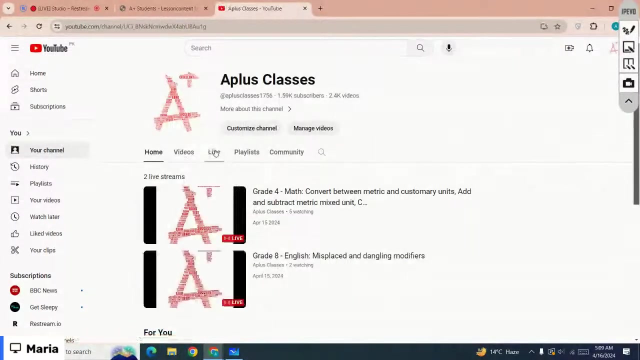 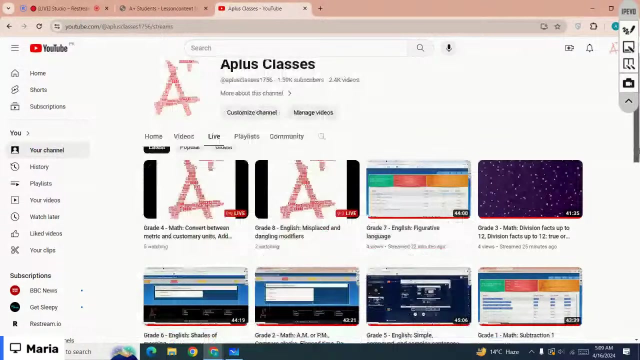 the same lesson again and again, but not- and no, I am not covering the same lessons. continue with the lessons from the next lessonюда hold on. let me just go to the. here is the channel. here is the live sessions. let me just show you the one we did in the last session before starting the new session. 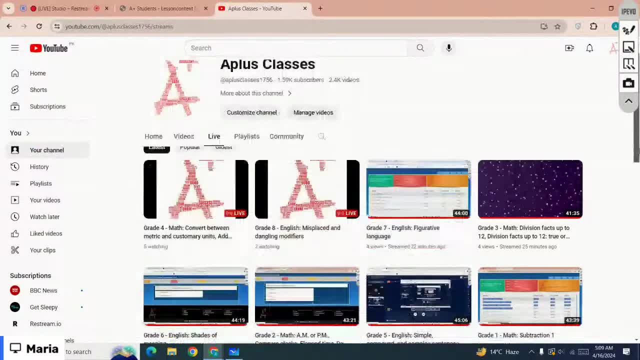 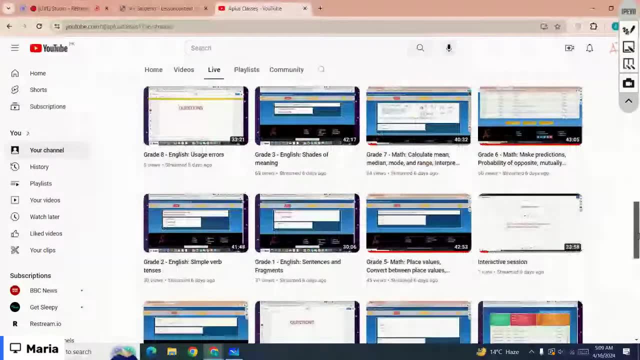 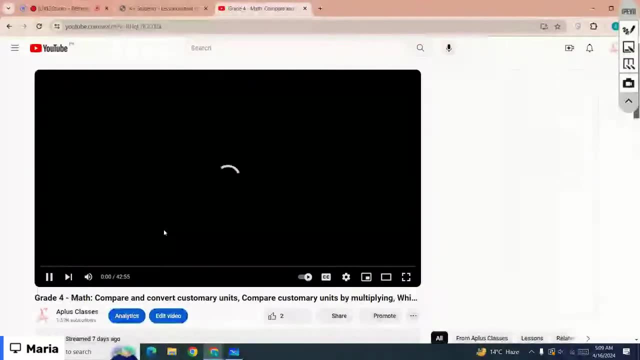 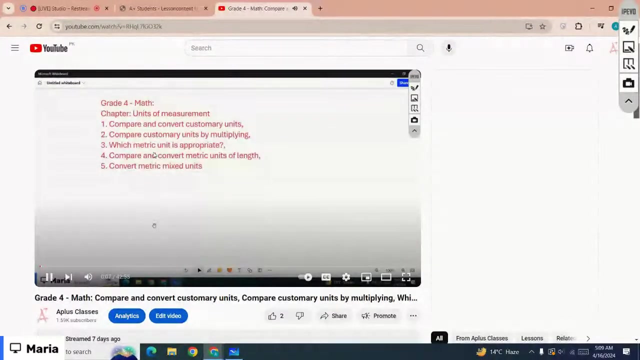 I always go and check for the one I did in the last week. never, ever, I repeated a session. here is the grade for session we did in the last week, right I. this is the compare and convert customary. these are the first five sessions from the same lesson we did in the last week right and before this session, let me show you the one. 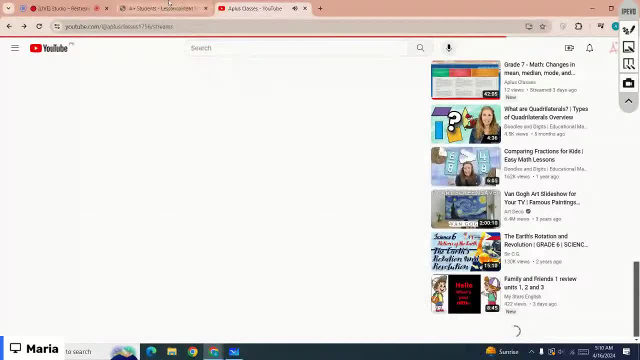 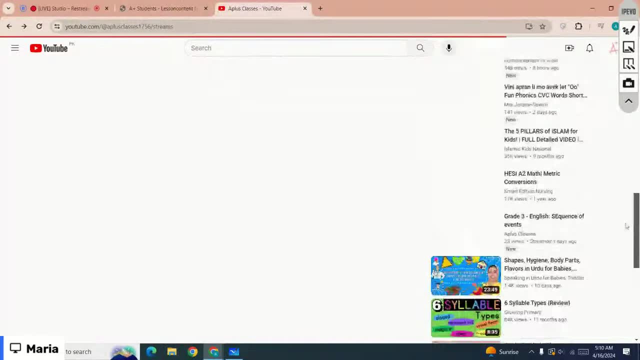 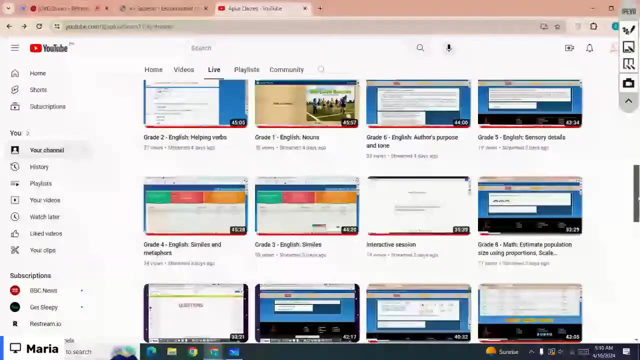 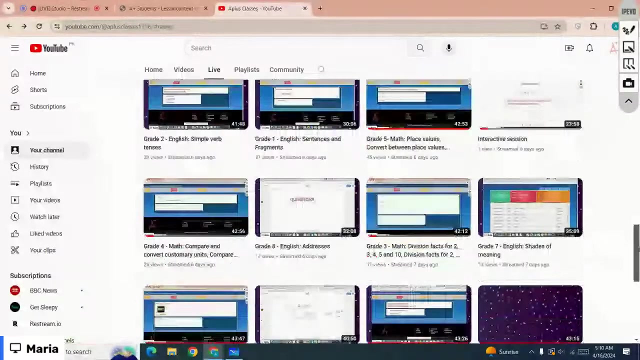 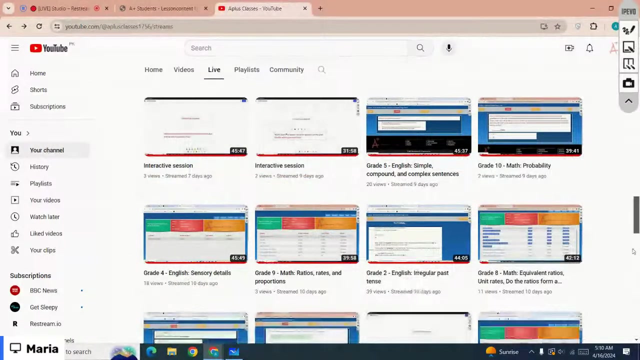 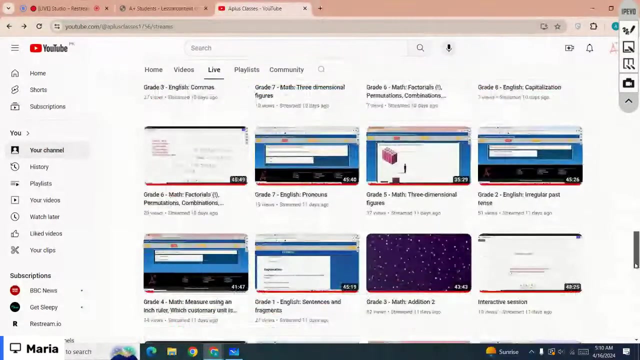 I did before this one, because I remember last time some of you made a complaint that I am. I am doing the same lessons again and again. here is the one I just showed. show you the one right, the one I did earlier before this one. they have the same names. that's why they seem you the same, but they are not same. here is the one. 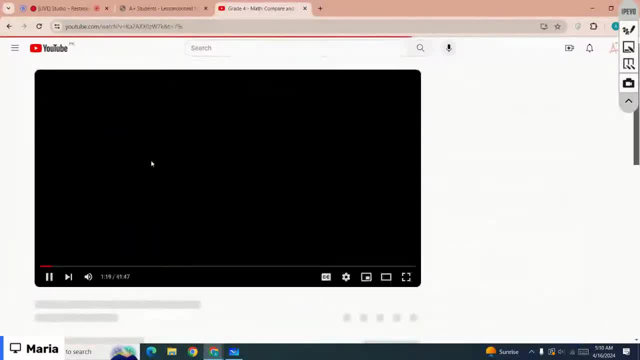 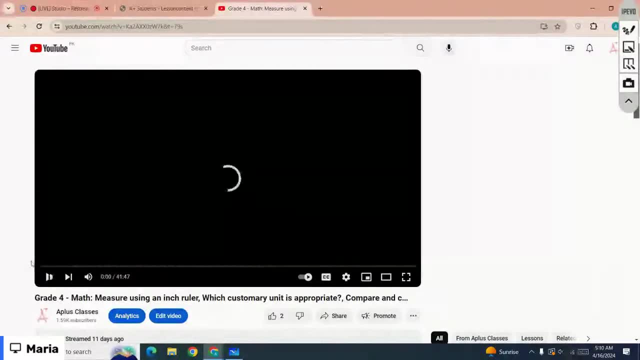 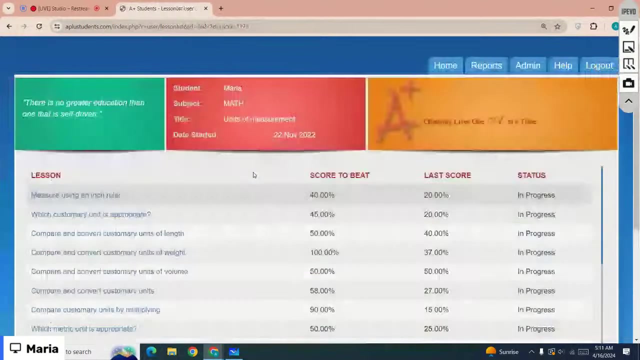 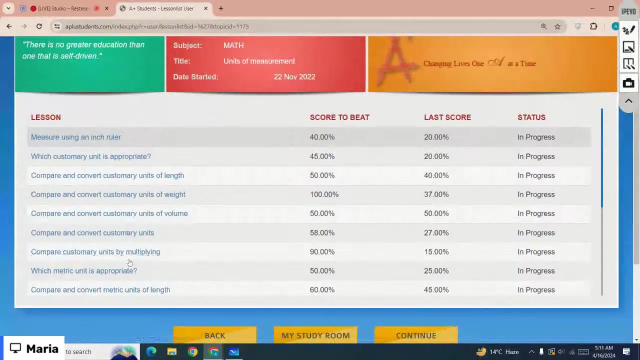 my ring inch ruler problem and the private lesson I will show you. I think you haven't checked Ablas on your own, and see, that is the one, the one I show you right now. then we covered this one, these four lessons, and now we are on failed. 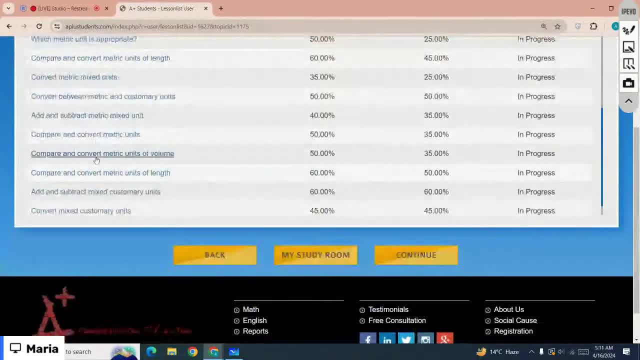 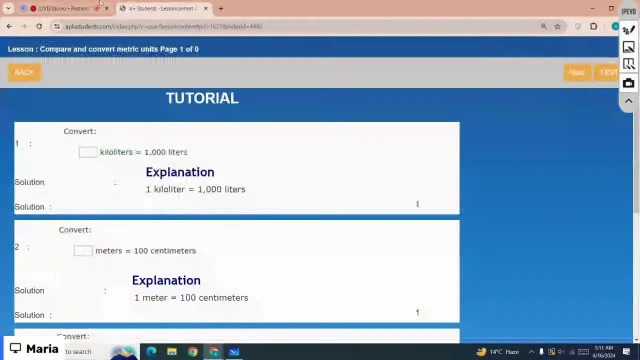 failed phantom, customary taste. e. we are here almost. we are almost on the ending, so they are not seen it. convert between metric and customer units. here I am. if you don't want to do then you can leave for tomorrow. you can join in the next session, next lesson: convert between: 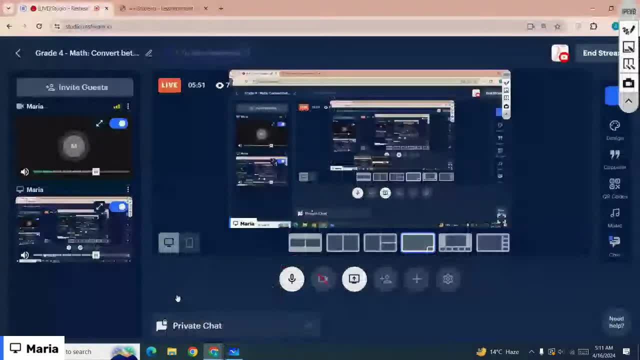 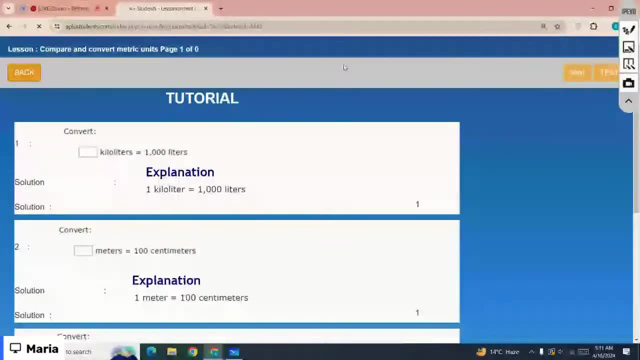 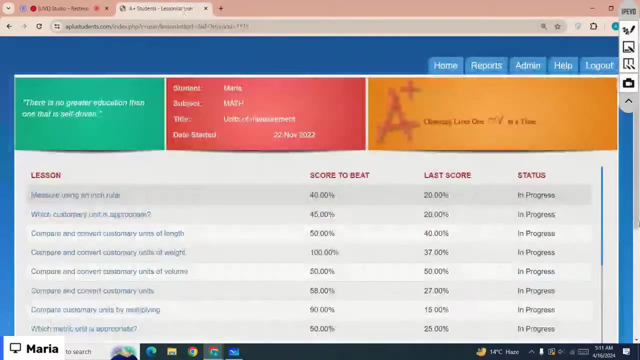 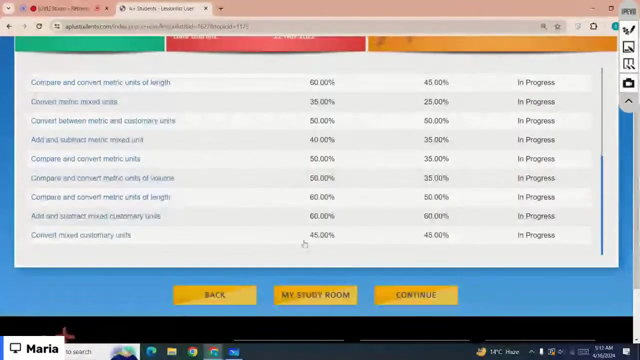 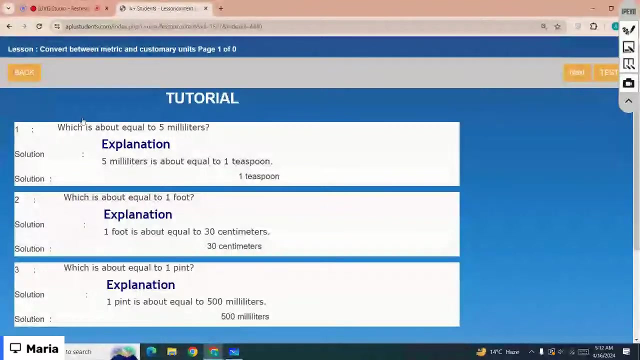 metric and customer units. they look same but they are not same. compare and convert, mmm, here is the one. compare, convert between metric and customer units, so which is about equal to five million milliliters. you have to see how they are equal, right? so five milliliters is about equal to one teaspoon, right? so five? 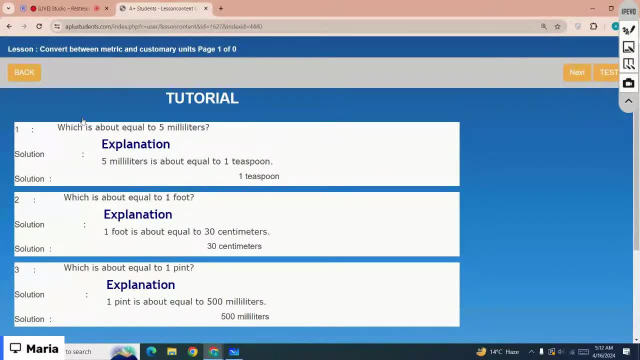 milliliters and one teaspoon. they both are exactly equal, which is about equal to one foot. so one foot is equal to 30 centimeters. they are just the basic units, right? so which is about equal to one pint, so which is the correct option. one pint is equal to: 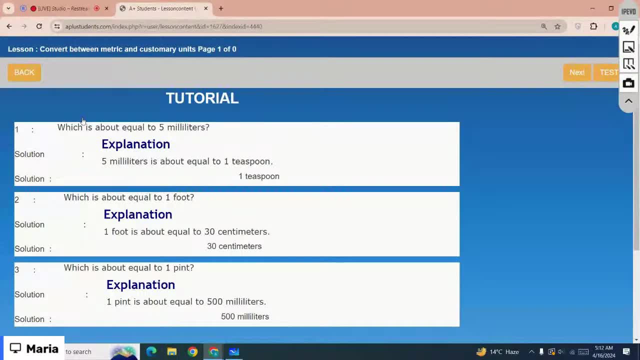 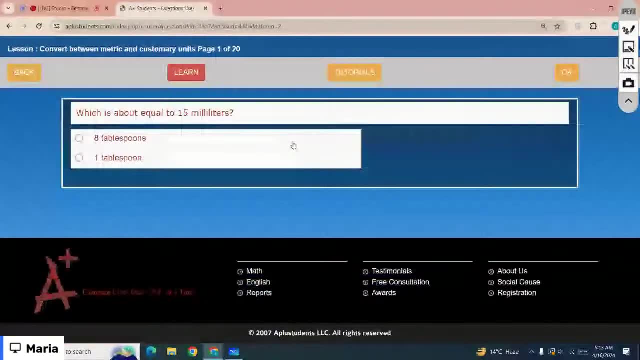 500 millimeters liters. let's just start with the test questions, which is about equal to 15 milliliters, which is the correct option. now let's see this rate. I am, the correct option is one tablespoon. 15 millimeter liters equal one tablespoon. 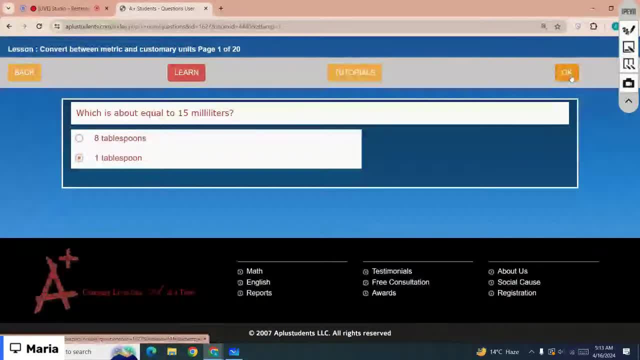 신, which is about equal to 3 feet, which is the correct option. 3 feet is equal to 1 meter. the correct option is 1 meter, which is about equal to 250 ml, which is the correct option. 1 pint or 1 cup. 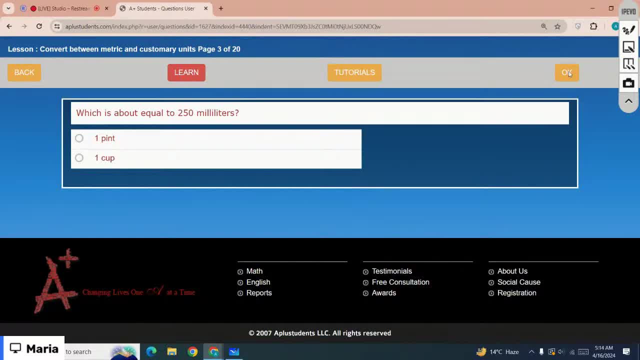 The correct option is 1 pint or 1 cup. The correct option is 1 pint or 1 cup. I think it's 1 cup. Yes, see, because 1 pint is very small, 250 ml must be 1 cup. 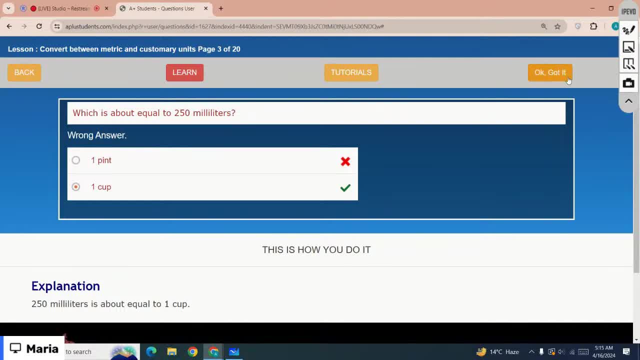 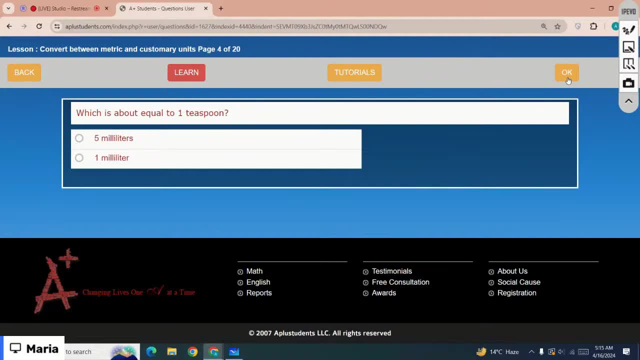 1 pint is too small, right. That must be 1 cup, Which is about 1 teaspoon, which is the correct option. That is 5 ml. The correct option is 5 ml, right, So I think it is a better option. 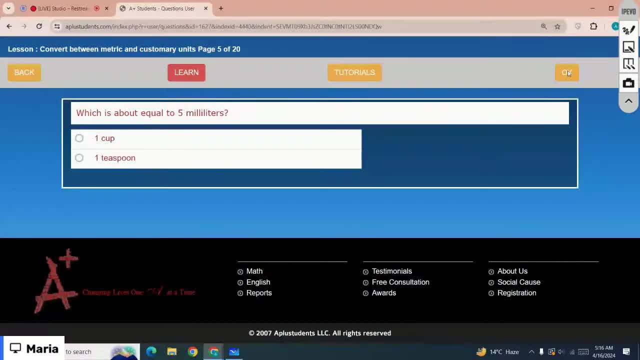 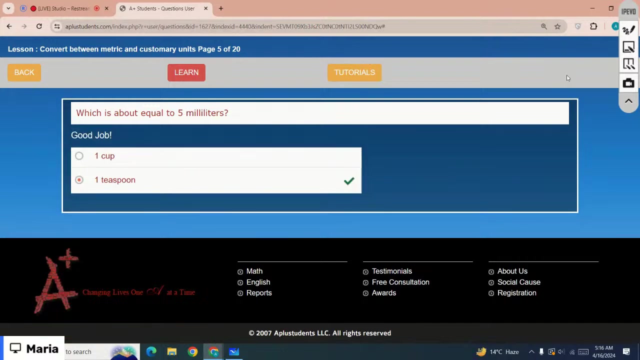 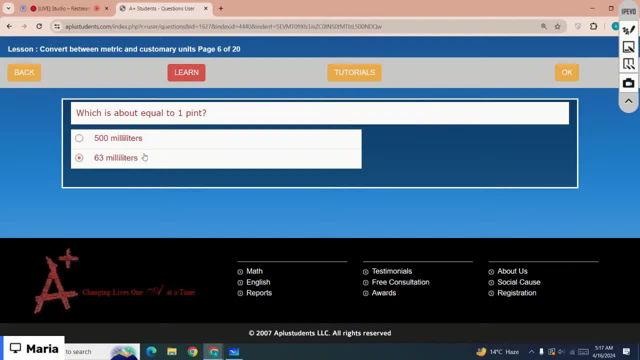 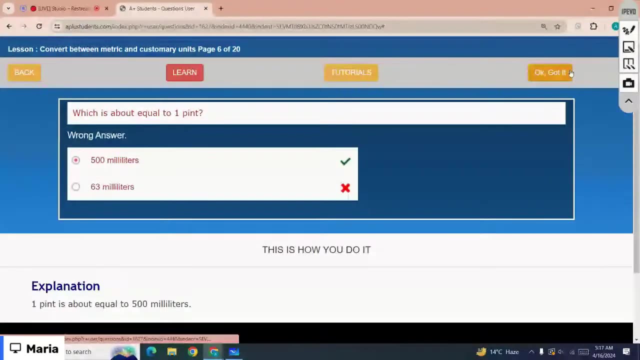 just did with 250 ml. 250 ml is one cup, so one pint is 63 ml. but it is a smaller, very small unit. the correct option is 63 ml. it is right. what's wrong with these questions? okay, you can complete the lesson by yourself later today. let me just move on to my 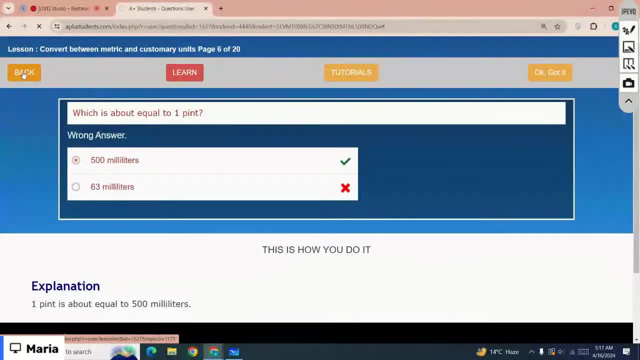 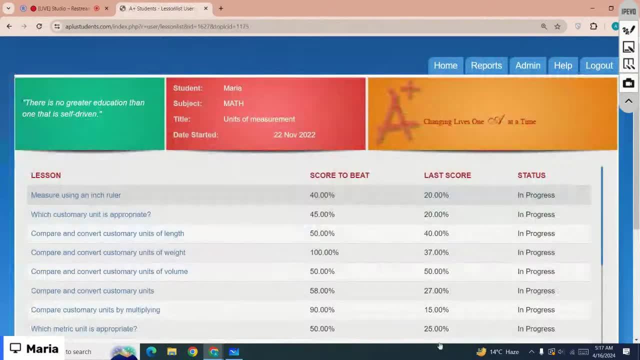 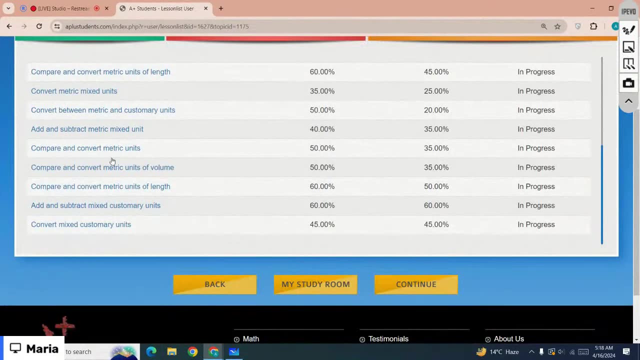 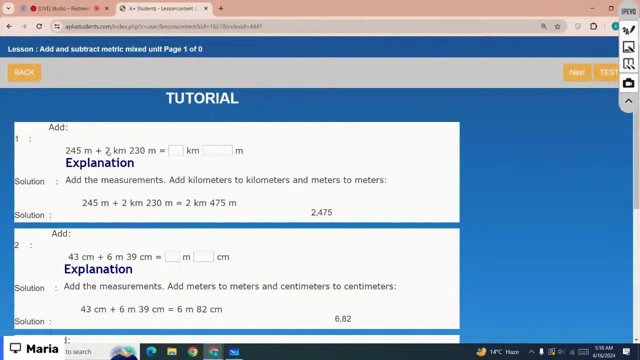 lesson and the next lesson is: add and subtract metric mixed units. then answer this question: add and subtract metric mixed units, okay, so you have to add 245 meters plus 2 kilometers plus 230 meters. you always add the same units, right? you add kilometers to kilometers and meters to meters, right? so you? 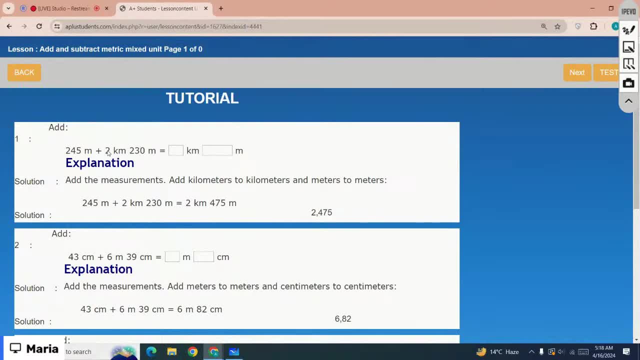 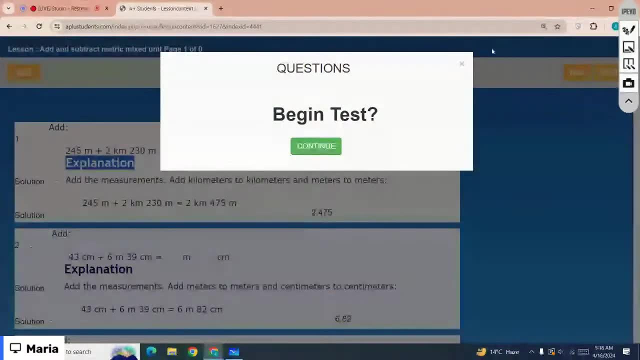 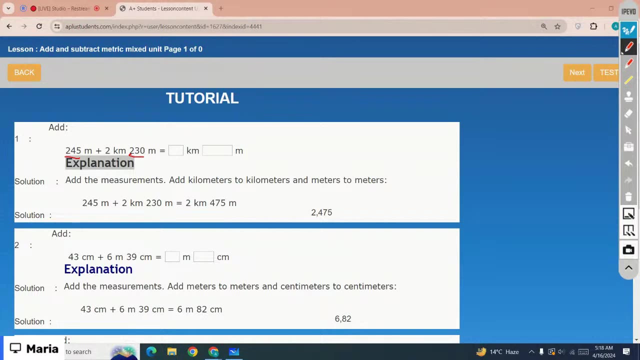 are not given with the kilometers here, with the first my value, so you just have the. you just have to add the meters, right? sorry, you can add 230 meter to 245 meter, right, that is 475 meters and two kilometer. you can write exactly same, so that would be two kilometer and 475 meters, got it? 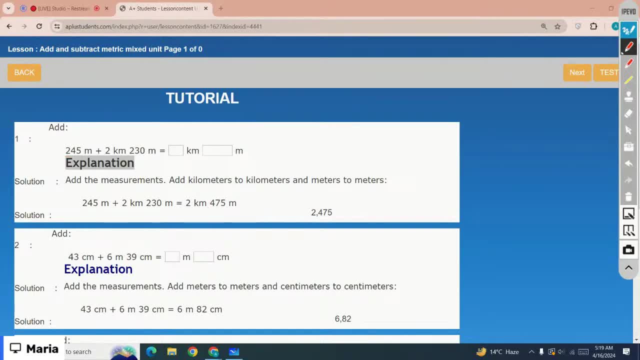 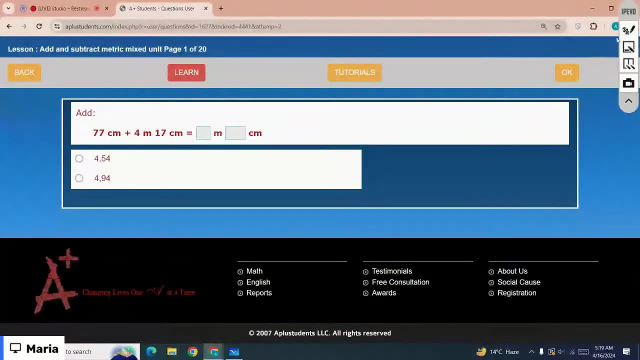 okay, let's just start with the test questions. okay, 77 centimeter plus 4 meter and 17 centimeter. right, so you will. you can add just centimeters to centimeters. so 17 and 77 is 7 plus 7 is 14. 4, 1 carry 7, 8 and 9, so you have 4 meters and 94. 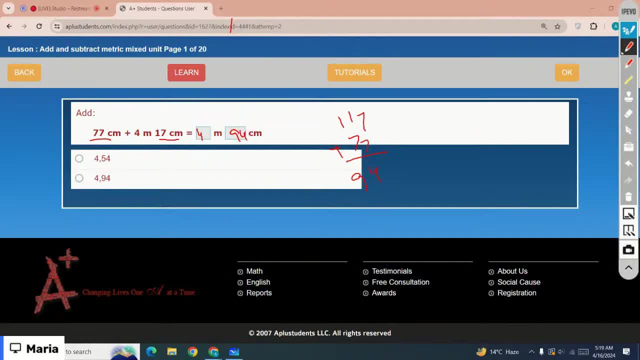 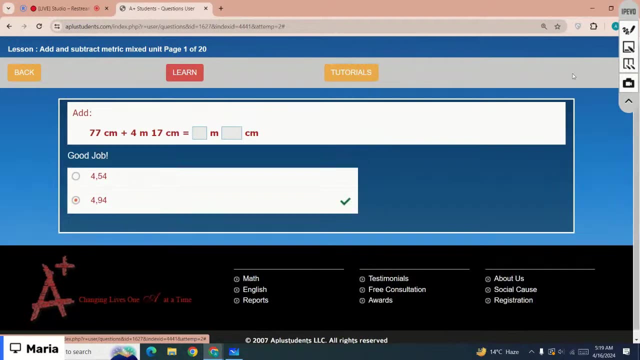 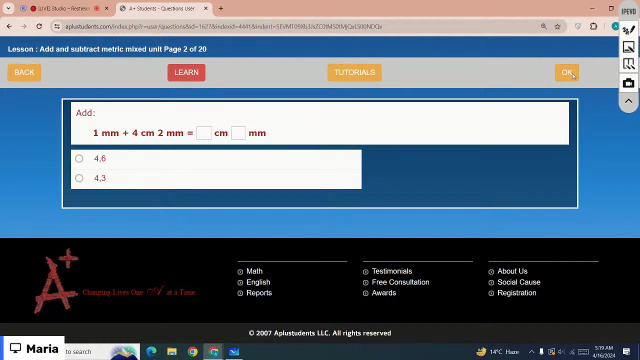 centimeters, got it. the correct option is 4 and 94. got it. option 2 is the correct option: 1 millimeter, 4 centimeter and 2 millimeter, which is the correct option. this is only. we'll add to the. we'll go. 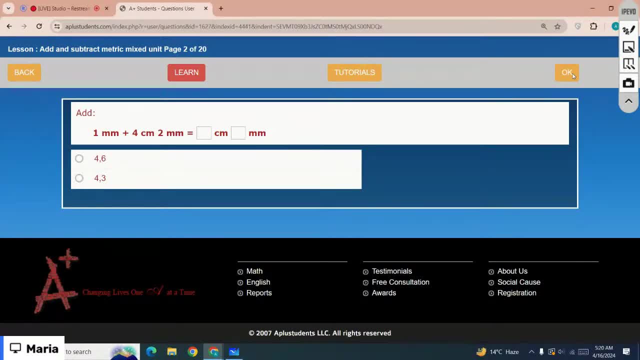 close. oh oh yeah. yeah, all right, we'll go into. yes, the correct option is four and three. very good, option number two is the correct option. the next one is three kilometer, 375 meter plus 594 meters, so which is the correct option? that is option number one. 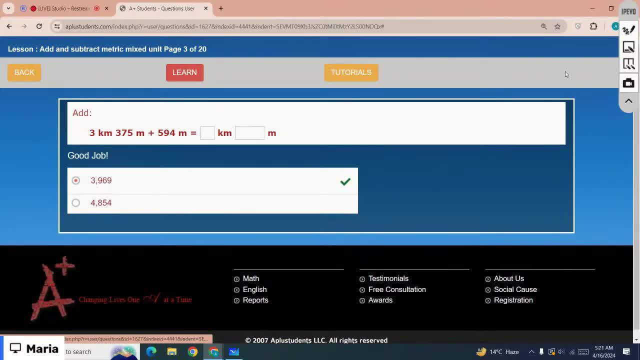 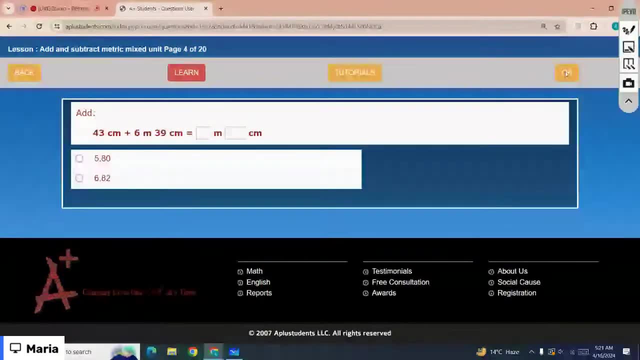 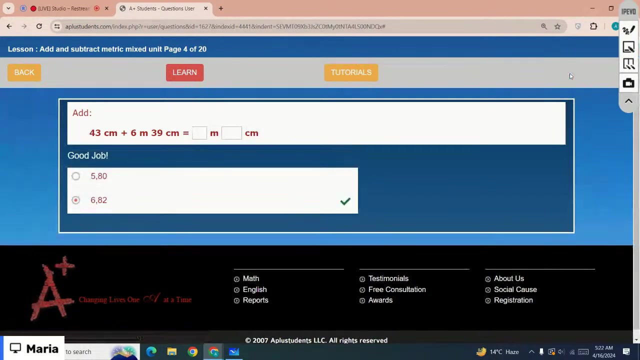 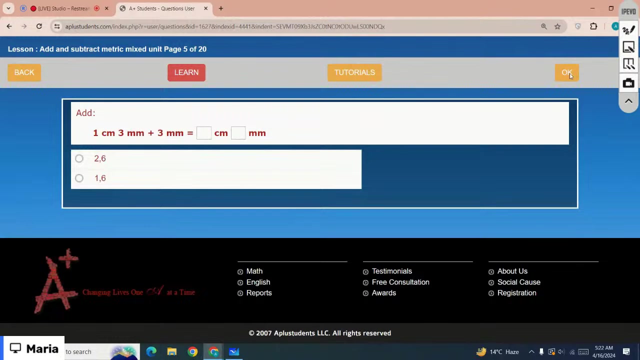 is the correct option. very good, 43 centimeter plus 6 meter and 39 centimeter. so which is the correct option? yes, that is the second option: 6 and 82 centimeter. one centimeter was three millimeter plus three millimeter, which is the correct option. 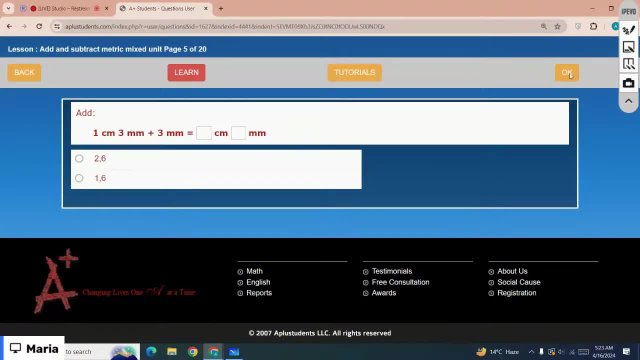 yes, that is one and six one centimeter, six millimeter. option two is the correct option. five millimeter, six centimeter plus two meter 43 centimeter, which is the correct option. yes, that is seven centimeter, 43 centimeter. option number two is the correct option right. 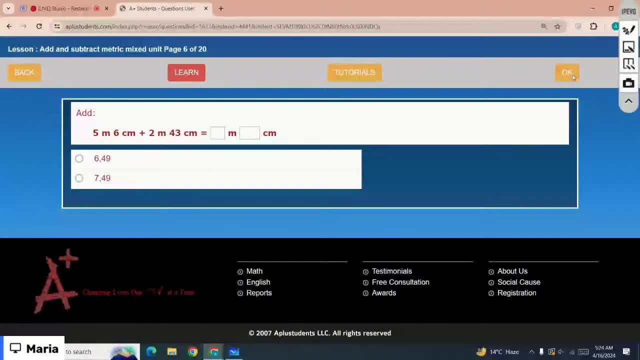 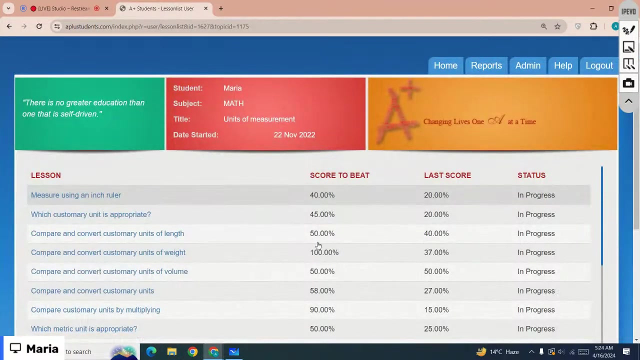 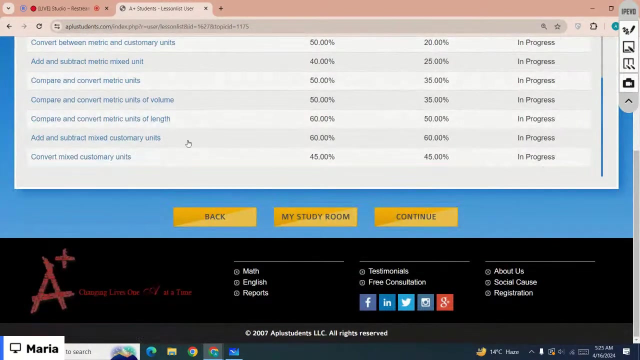 option number two is the correct option. okay, you can complete the lesson by yourself later today. let me just move on to next lesson. okay, you can complete the lesson by yourself later today. let me just move on to next lesson. the next lesson is convert. makes no compare and convert metric units. 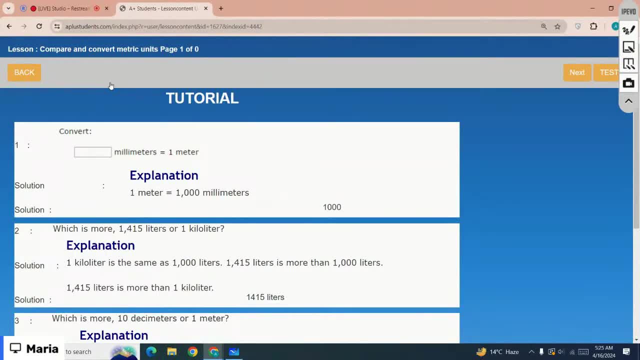 okay, one meter equal how many millimeters? okay, one meter equal how many millimeters? one meter equal one thousand millimeters. one meter equal one thousand millimeters. one meter equal one thousand millimeters. millimeters, right, which is more? 1 kilometer or 1415 liters, 1 kiloliter. 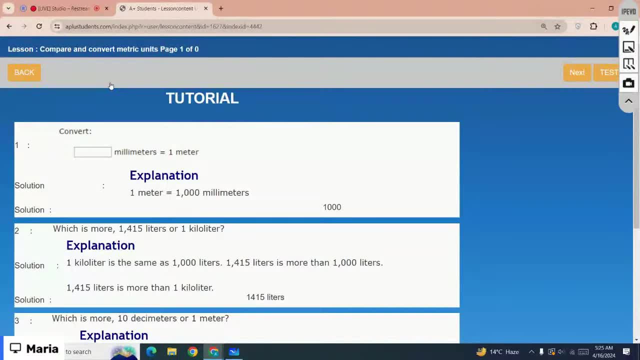 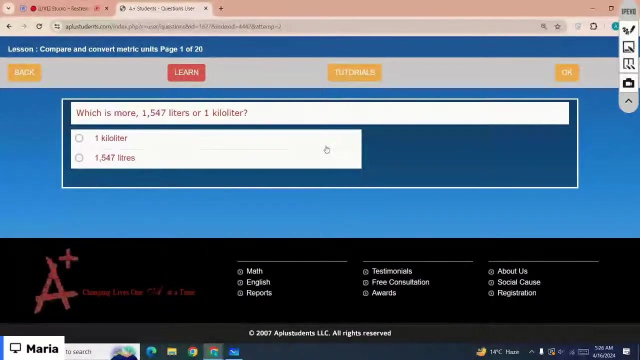 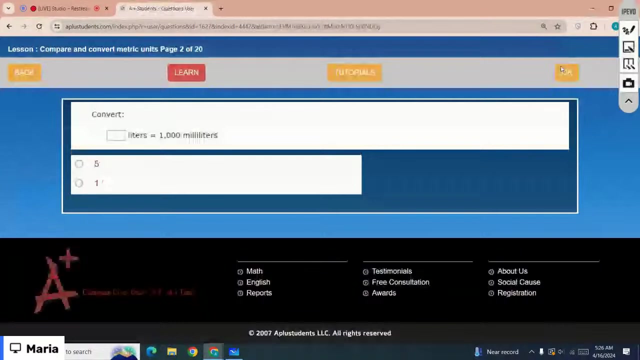 equal 1000 liters, right? let's start with the test questions: which is more, 1 kiloliter or 1547 liters, which is more? the correct option is: one thousand 547 liters is more right. option number 2 is correct: 1000 milliliters equal- cool gil. 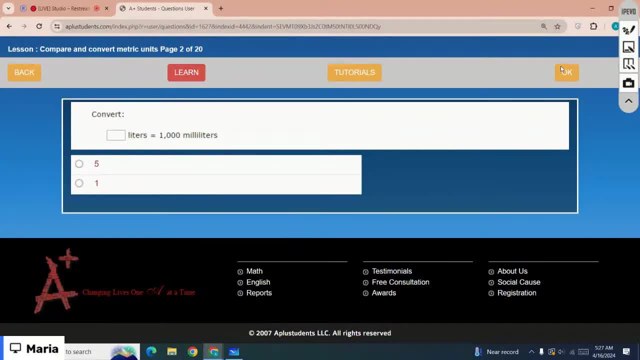 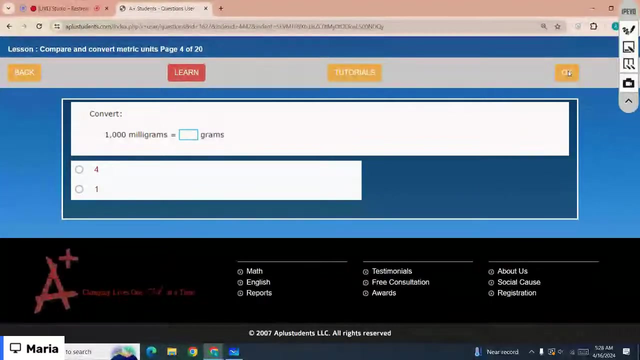 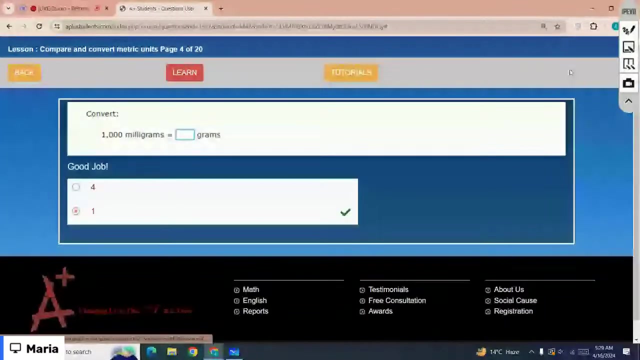 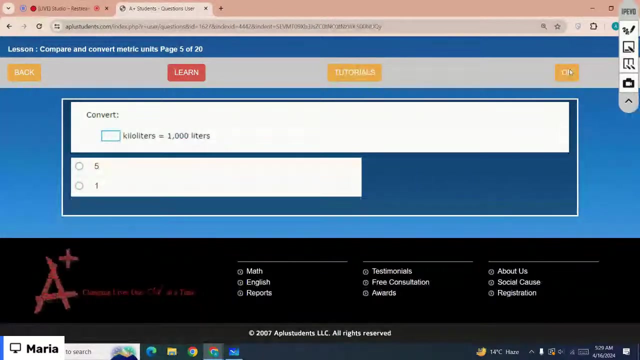 how many liters? yes, that is one liter. the correct option is one 1,000 grams equal. how many kilograms? yes, 1 kilogram. it is 1,000 milligrams equal. how many grams? that is one gram? the correct option is one one thousand liters equal. how many kilograms? 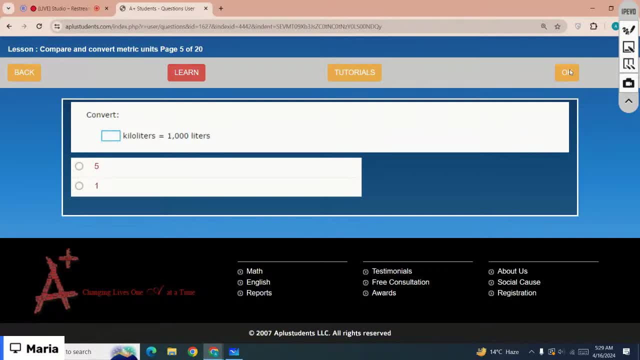 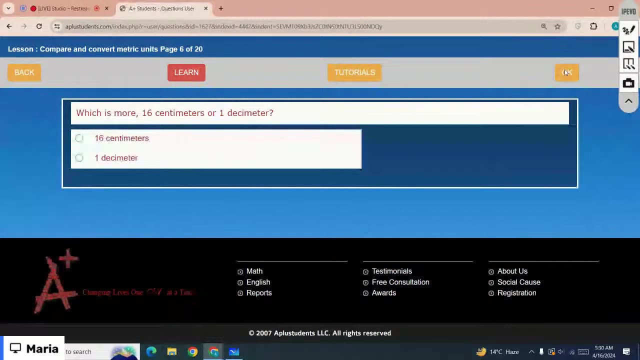 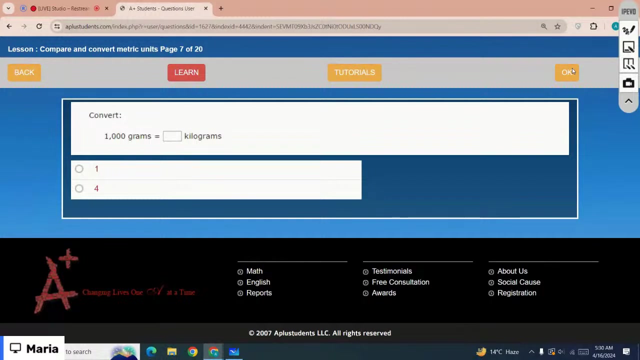 youín, that is one kilometer, which is more, 16 centimeter, or one decimeter, which is the correct option. so 16 centimeters, because in one decimeter you have 10 centimeters. 1000 grams equal how many kilograms? the correct option is one kilogram, right. 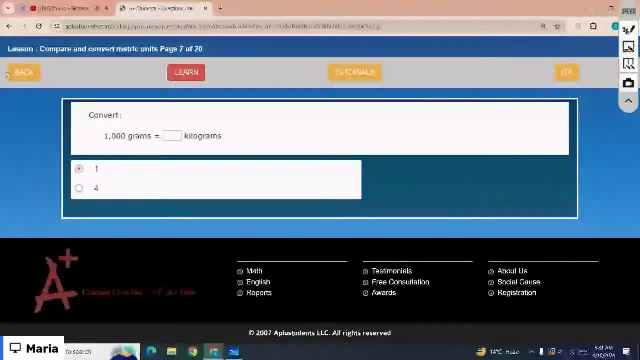 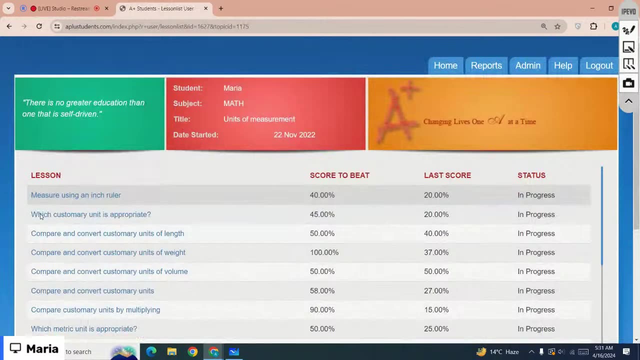 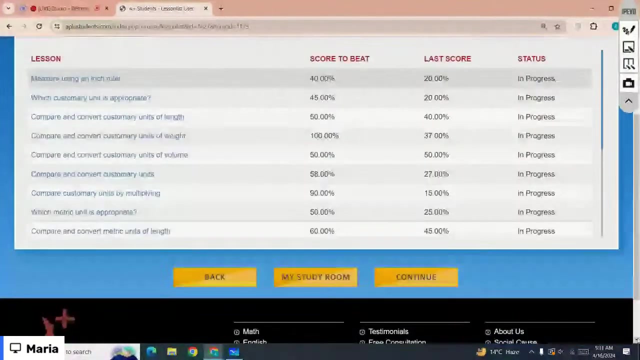 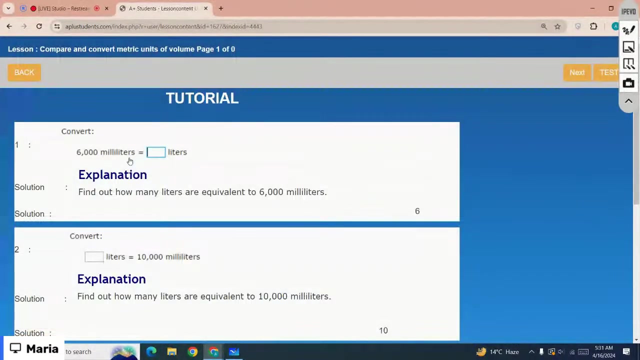 okay, you can complete the lesson by yourself later today. let me just move on to next lesson, which one equal? the next lesson is compare and convert metric units of volume. okay, six thousand milliliters equal how many liters s? let's do other exercise: one liter equal one thousand milliliters, right? so then, six thousand milliliters equal pocket making of 100 milliliters. another liter equal 1000 milliliters, right? so then, six thousand milliliters were necklace and sı varıç k Support Ne gimmicks. 1 liter also equal 1,100 ml. as a price of a liter, then편 BB2. total price we divide by долar Line: ăr ışık nedirło 2,3artıs. plus 1 liter equal 1000 ml. I always skip 2,. 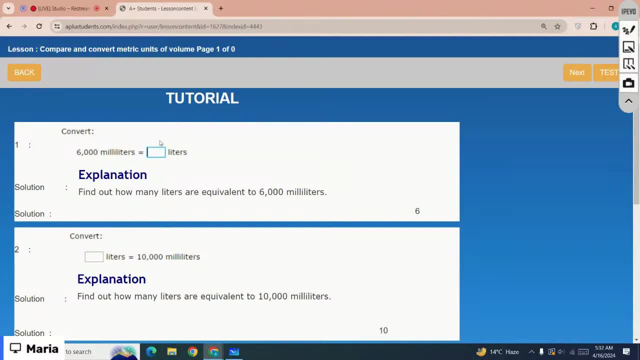 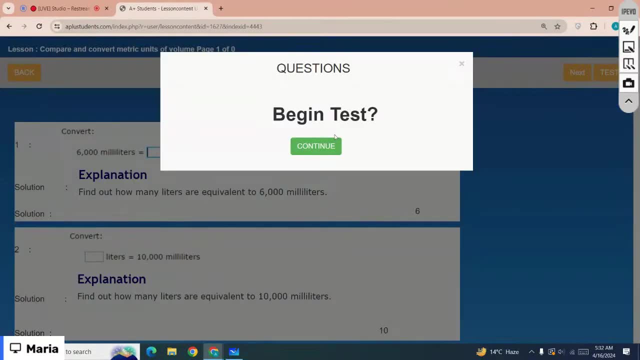 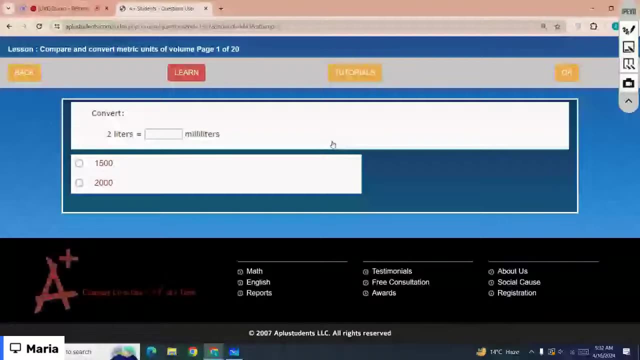 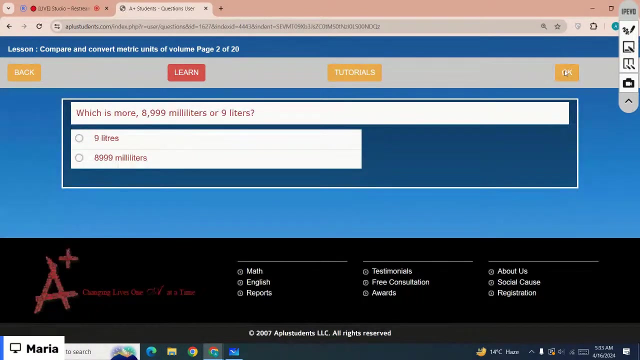 is equal six liter. Let's just start with the test questions: Two liters equal how many milliliters? Two liters equal two thousand milliliters? option number Two is the correct option. Which is more eight thousand nine hundred ninety nine milliliters or nine liters, Which? 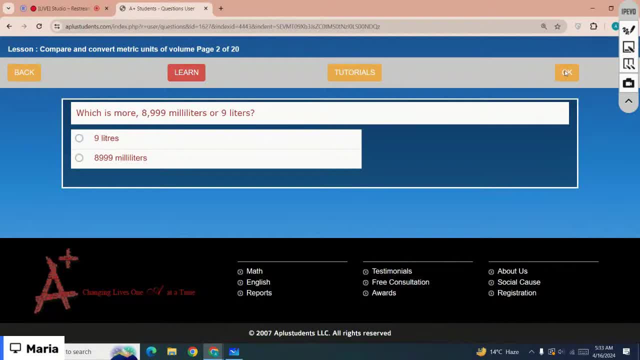 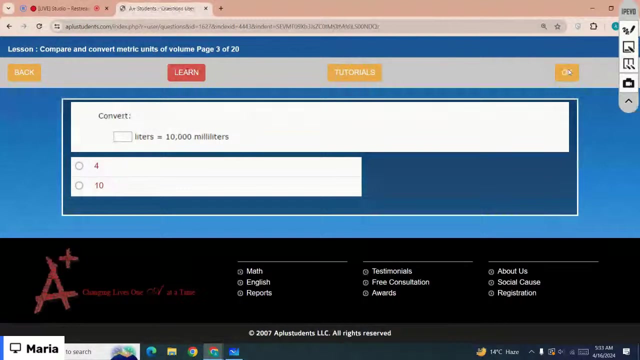 is the correct option. In nine liters you have nine thousand milliliters, right? So nine liters is more Ten thousand milliliters. Example: What is the best direction? of Omega: letting you do長itization. Double-reflective mass. 10,000 milliliters. Yeah, Fiveoughing or gSI. Two liters equal nine thousand milliliters or 9,000 milliliters. Which is the correct option? Does it make sense? What kind of reaction? Do we know data? 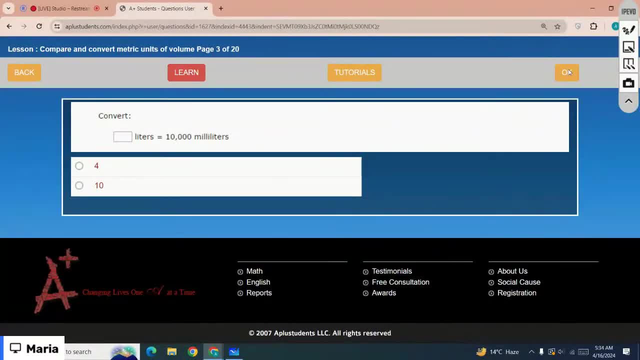 Rigth, Good, good job, We have all right. Then, if we do gSI, if not다는melceloran, with all these things, what is the situation? 10,000 mL is equal to how many liters, That is, 10 liters. 10,000 mL is equal to 10 liters. 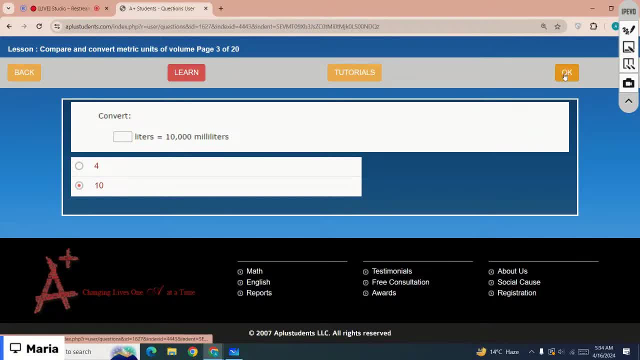 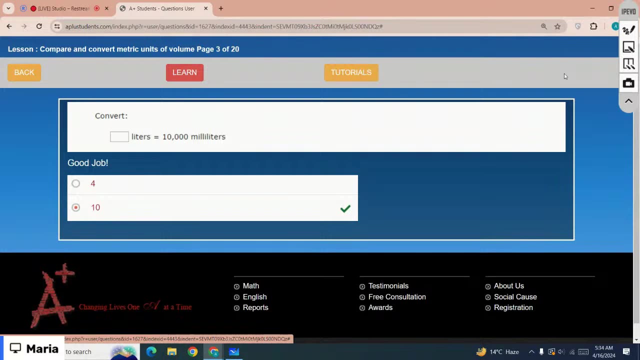 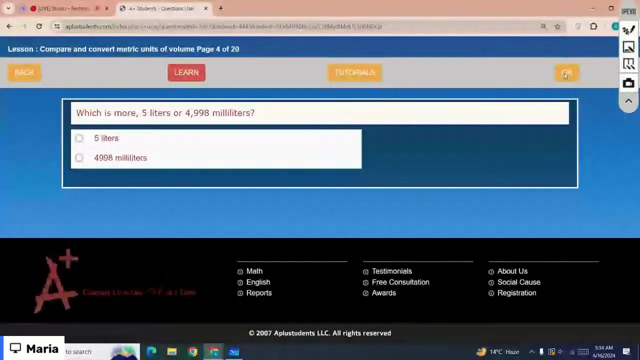 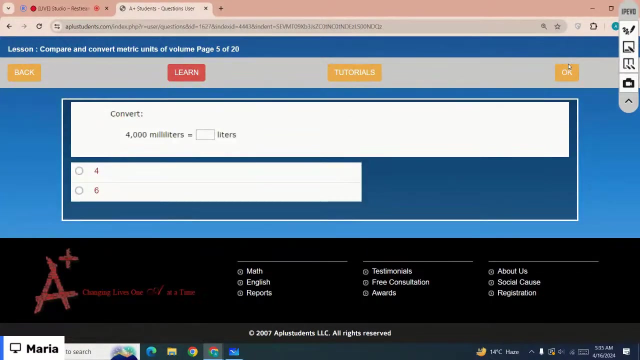 Very good, Okay. the next one is: which is more: 5 liter or 4,998 mL? 5 liters is more. the correct option is 5 liters. We convert: 4,000 mL is equal to how many liters. 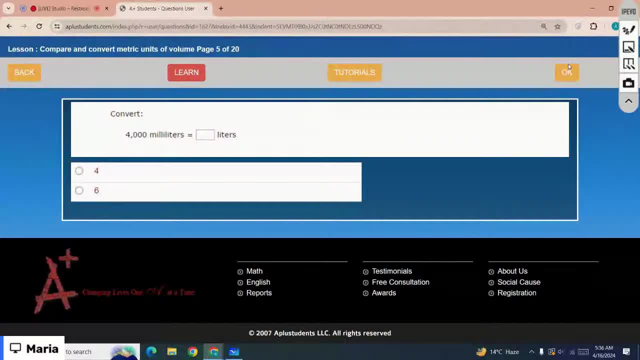 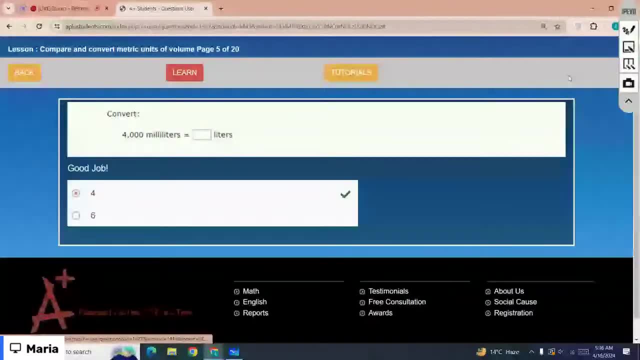 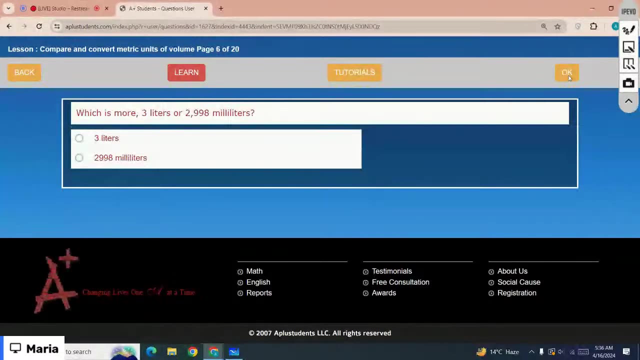 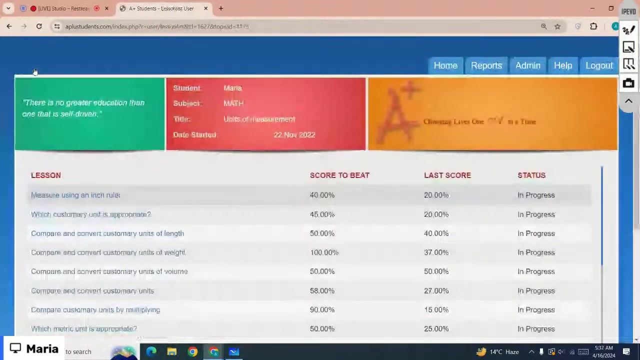 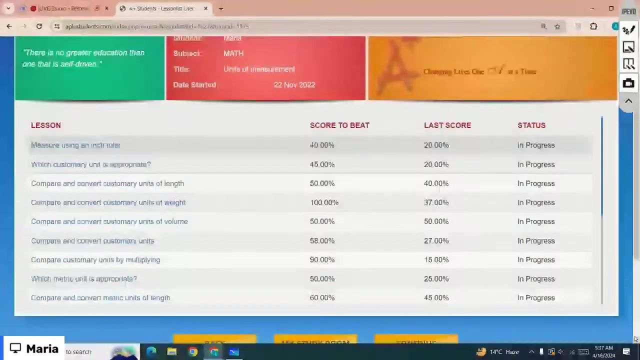 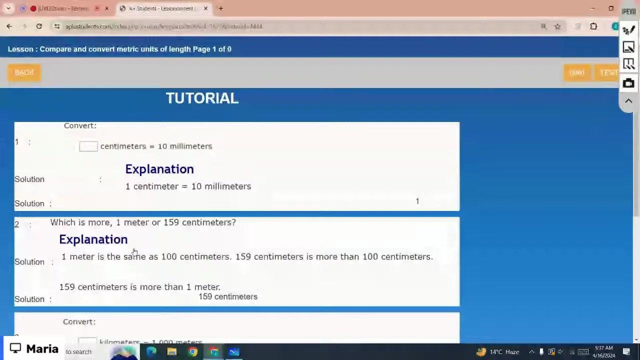 That is 4 liters. the correct option is 4.. Okay, you can complete the lesson by yourself later today. Let me just move on to the next lesson. The next lesson is compare and convert metric units of length. 10,000 mL is equal to how many centimeters? 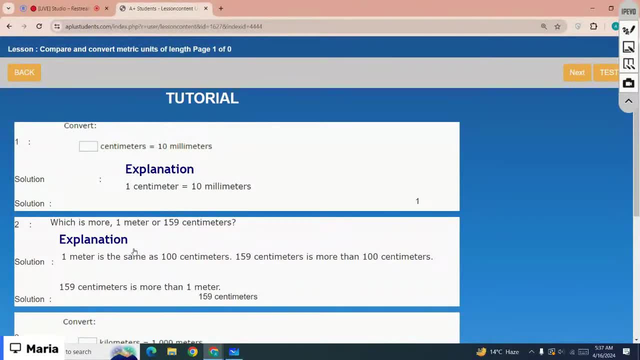 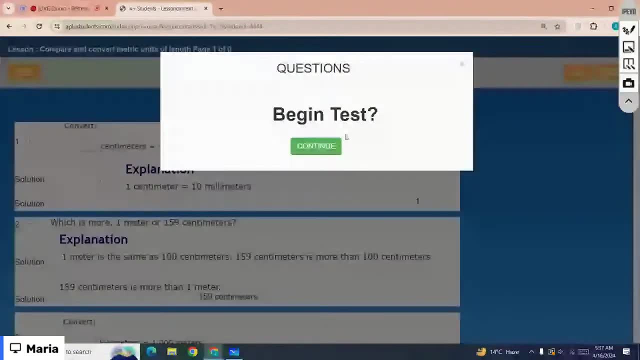 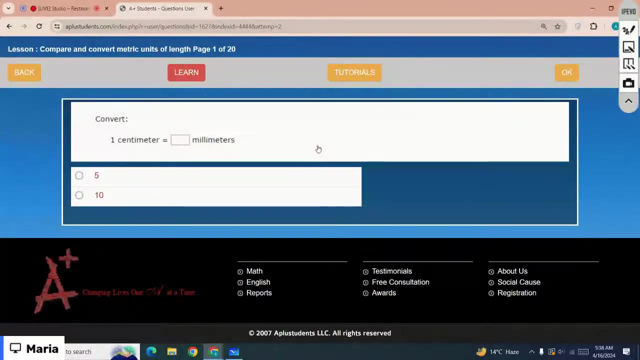 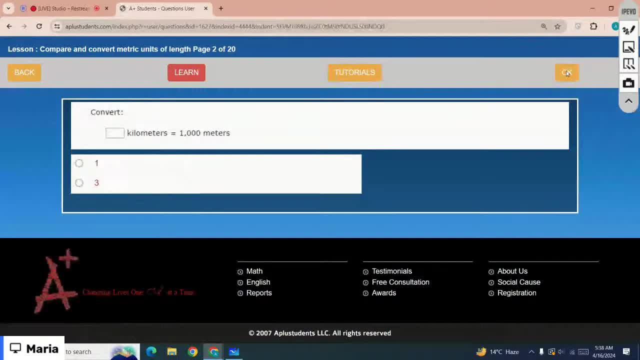 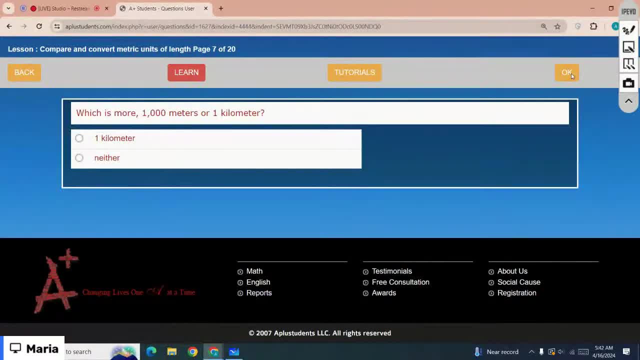 thousand meters or one kilometer. the correct option is 930, because they both are exactly equal. okay, you can complete the lesson by yourself later today. so we were working on grade 4 math. the chapter we working on is: you don't have my a mint. we're going to start the next lesson in the next 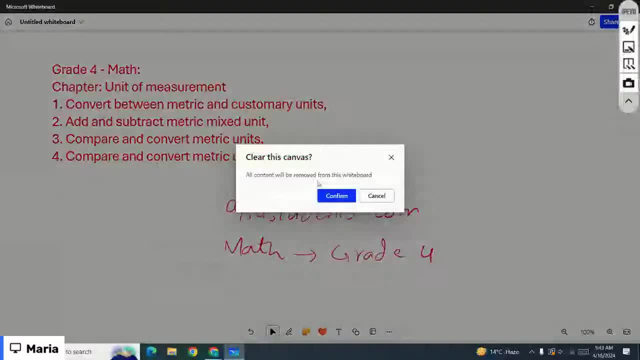 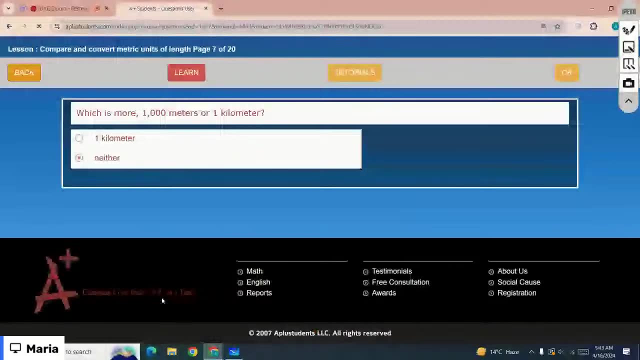 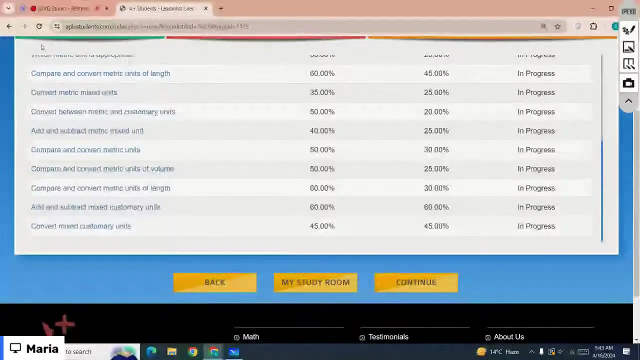 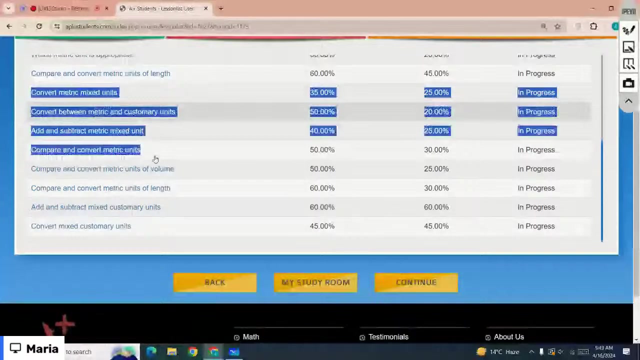 session. next chapter in the next session: right, so the lessons we have got today are: can compare and convert, convert. convert metric mixed unit. compare and convert metric and customer units. add and subtract mixed units. compare and convert metric units. compare and convert metric units of volume and compare and convert metric units of length. so please make. 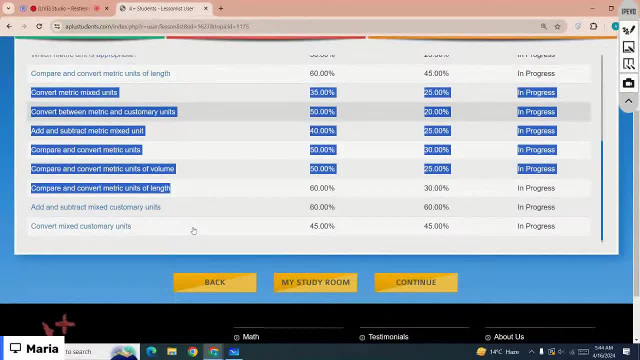 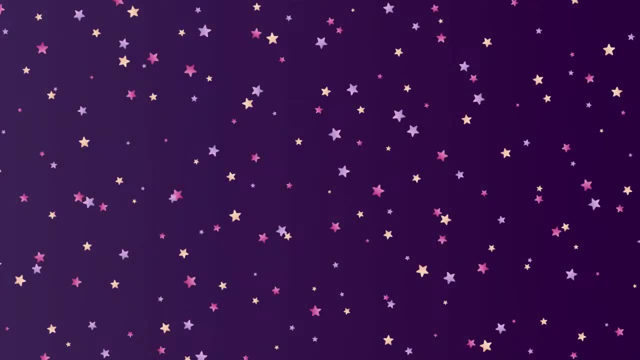 sure, before the next session you can complete all the practice questions for the lessons we did today. that is your homework until next session, right? and so if you need more help with any of the lesson, you can contact any tutor on the Skype. they are available from Monday to Friday, five to nine, or either you can. 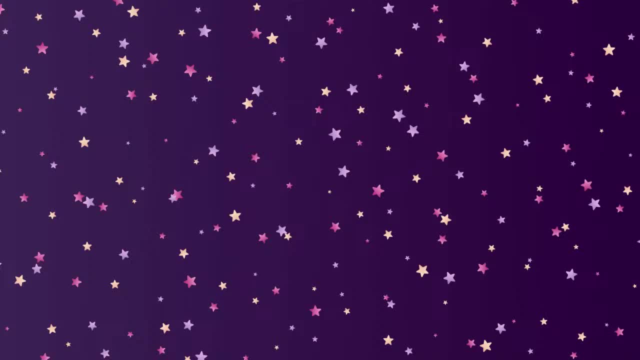 join me in the interactive session. that would be daily from four to five and from nine to ten. so that's all for today. if you have any questions- literally lesson we have just finished- you can please ask. I'm here to answer all your questions and confusions, if you have any. 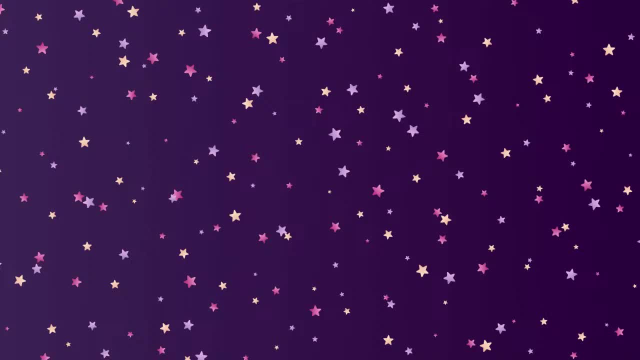 questions or questions. please feel free to reach out to me, and my msd is tindaythah on the Skype. that is available on the Skype. it also has a link to my email address to the website, where you can find all the information that we have. 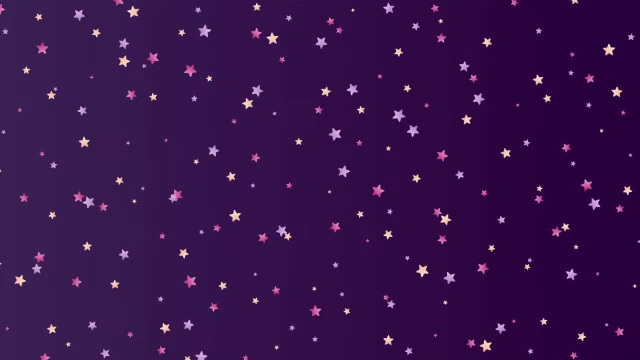